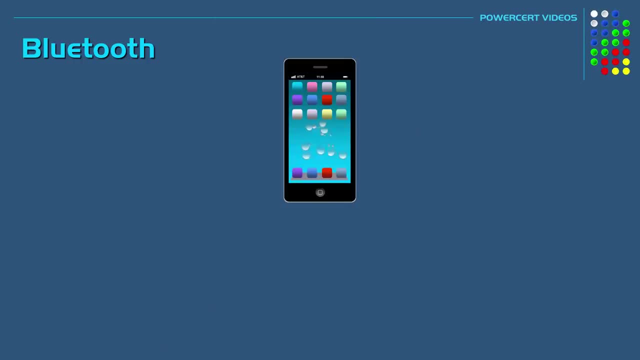 exchange information and protect each other. Any activity that is connected to the tablet will be wirelessly connected to a Bluetooth or wireless device that is connected to the wireless device information between them. Now, the most common use for Bluetooth is for wireless audio streaming, such as pairing. 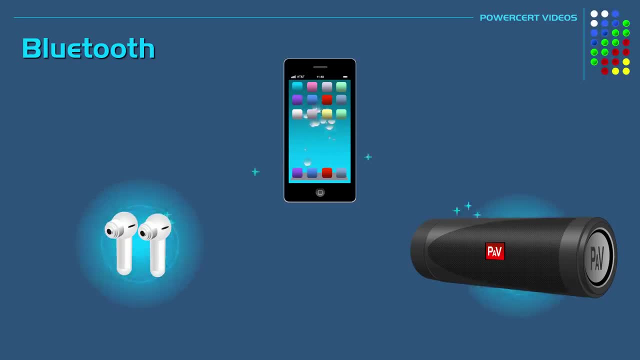 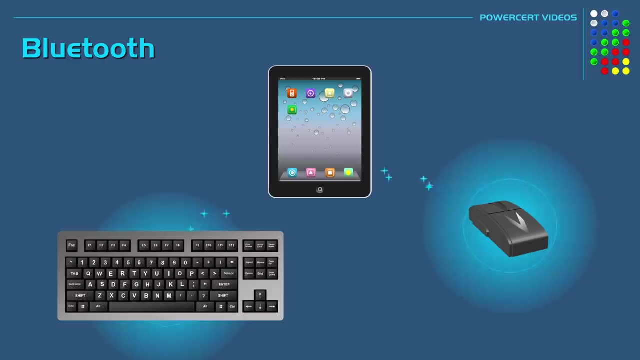 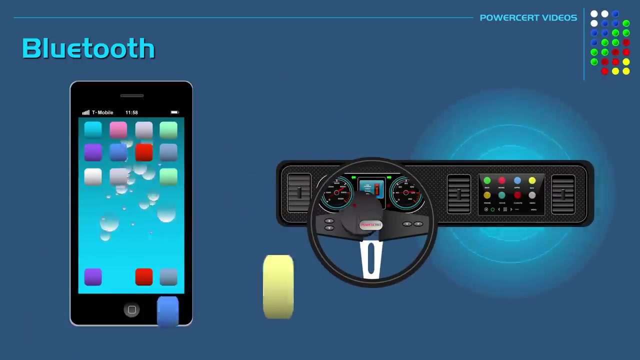 your cell phone to wireless earbuds or an external speaker. It can also be used for pairing headphones to a TV or pairing a wireless keyboard and mouse to a tablet or computer, But one of the most common uses is pairing your cell phone to your car's audio system. 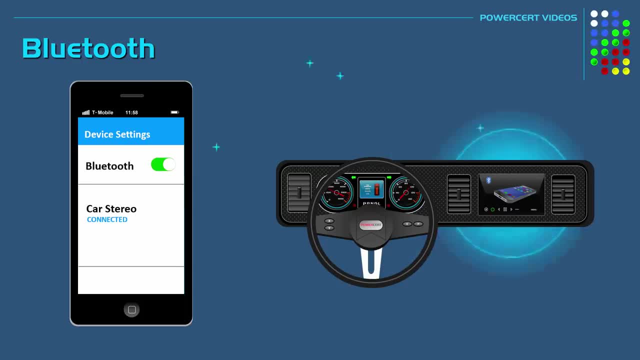 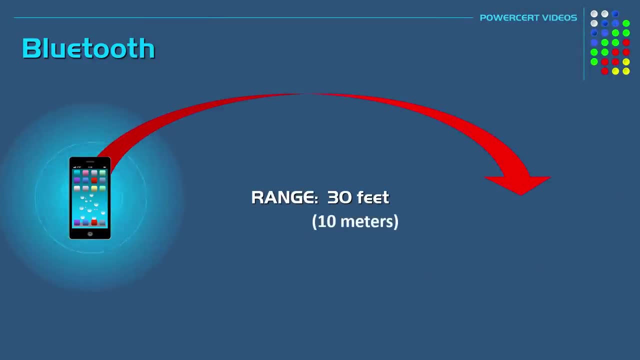 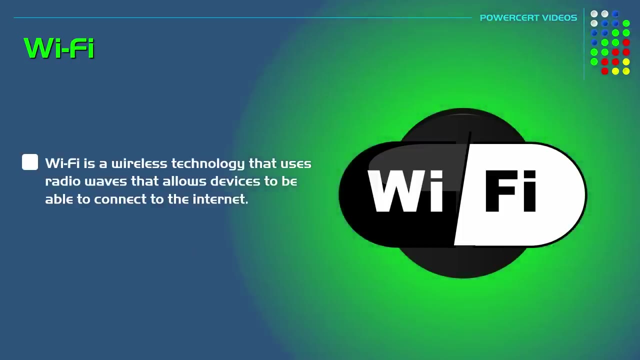 which enables hands-free use when you're on the phone while driving, And the range of Bluetooth is approximately 30 feet or 10 meters. Now let's talk about Wi-Fi. Now, Wi-Fi is a wireless technology that uses radio waves. that allows devices such as desktop. 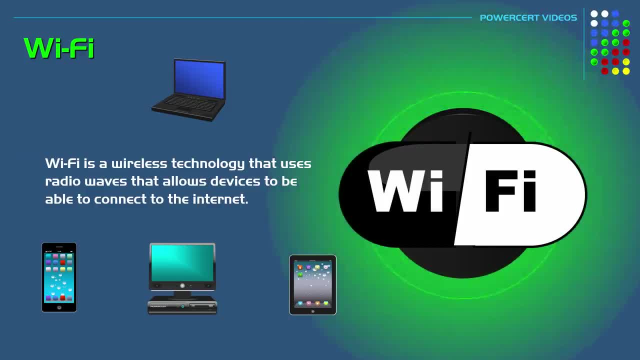 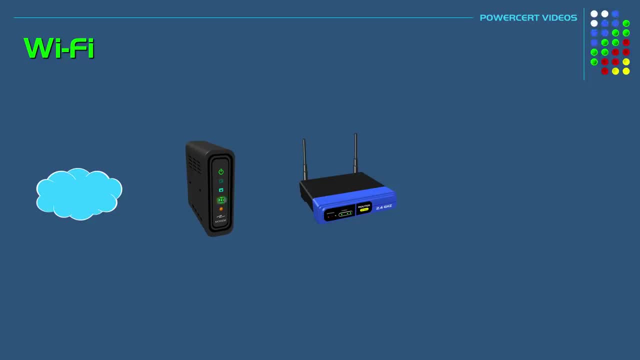 computers, laptops, tablets and cell phones to be able to connect wirelessly to the internet, And the most common way that Wi-Fi devices access the internet is by connecting to a Wi-Fi router. Wi-Fi routers will have a connection to an internet service provider that will broadcast. 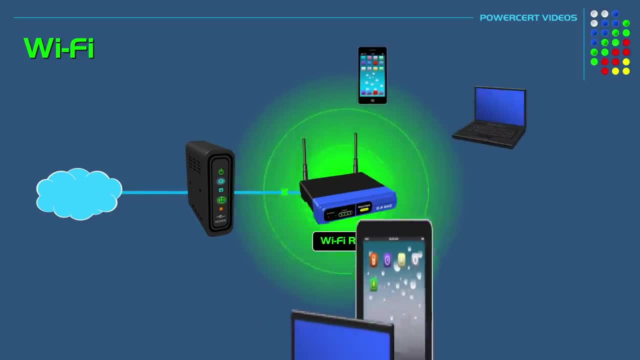 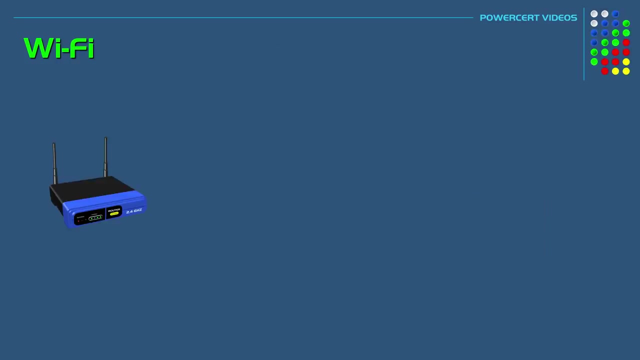 a Wi-Fi signal so that nearby devices can connect to the signal and grant them internet access. And in addition to internet access, these devices can be configured to exchange information between them by creating a network And depending upon the surrounding environment. Wi-Fi has a range anywhere from: 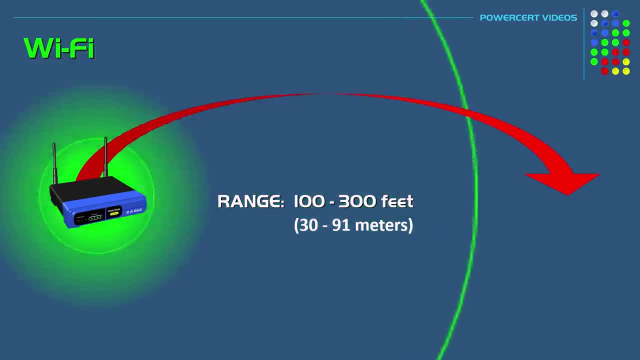 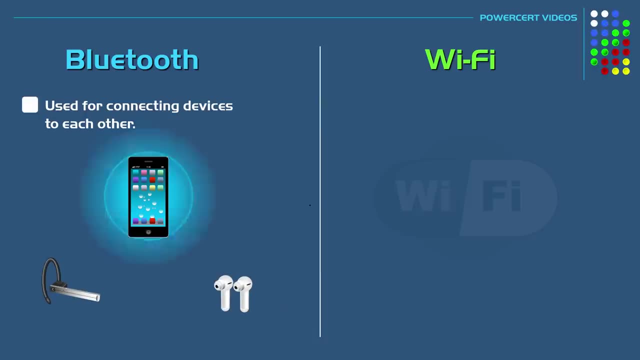 100 to 300 feet. So what are the differences between Bluetooth and Wi-Fi? Well, the main difference is that Bluetooth is for connecting devices to each other to exchange data And Wi-Fi is used to connect devices to the internet. And another difference is range and speed. 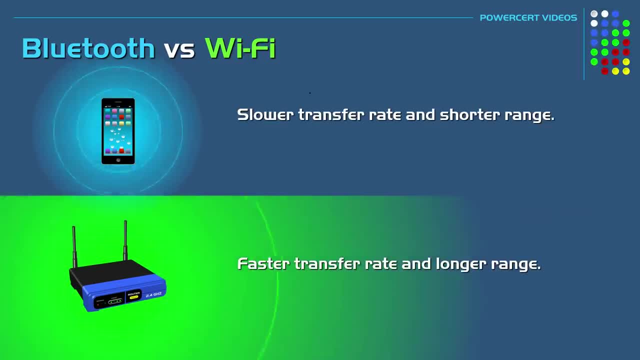 Bluetooth has a slower transfer rate and a shorter range, And the main reason for this is power. Bluetooth uses less power than Wi-Fi, So, even though it sacrifices in range and speed, it also has an advantage with longer battery life, with less frequent charging, which allows Bluetooth devices to be manufactured. 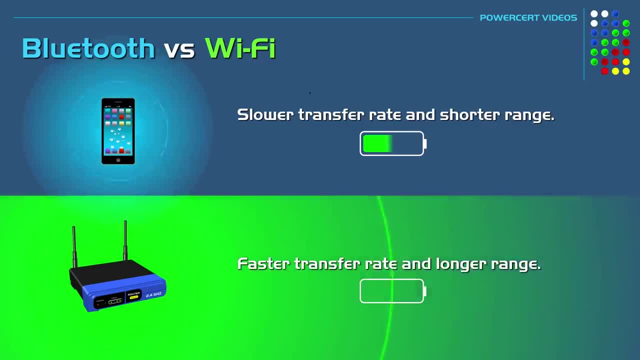 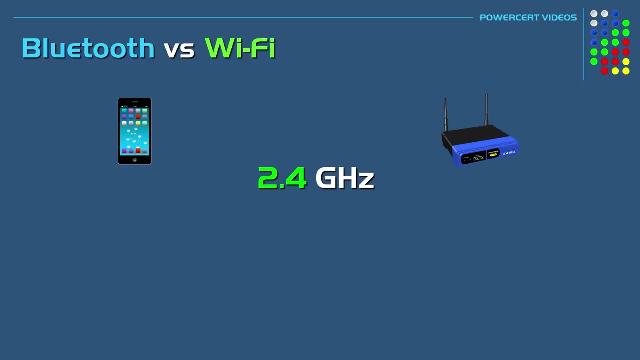 in a smaller size that doesn't require large batteries. But Wi-Fi, on the other hand, is faster than Bluetooth and has an approximate 10 times longer range. Now, both Bluetooth and Wi-Fi operate at 2.4 gigahertz, But the thing is, a lot of other devices operate at 2.4 gigahertz.